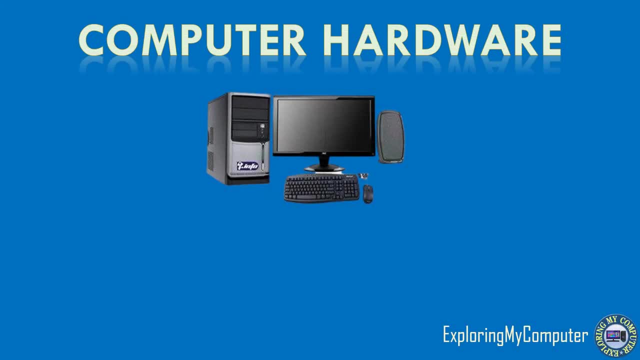 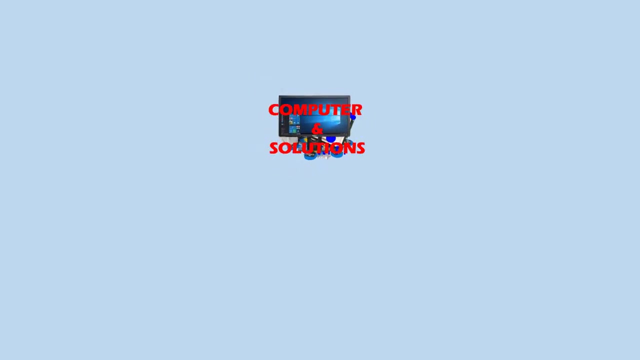 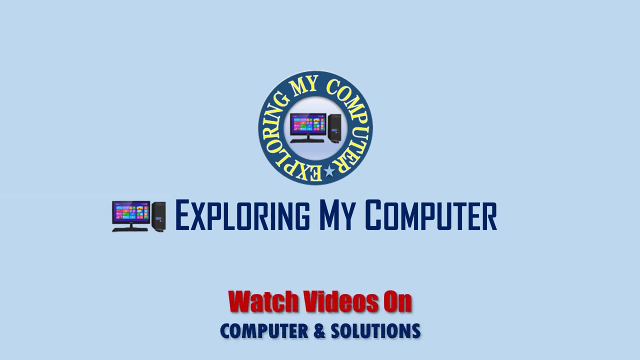 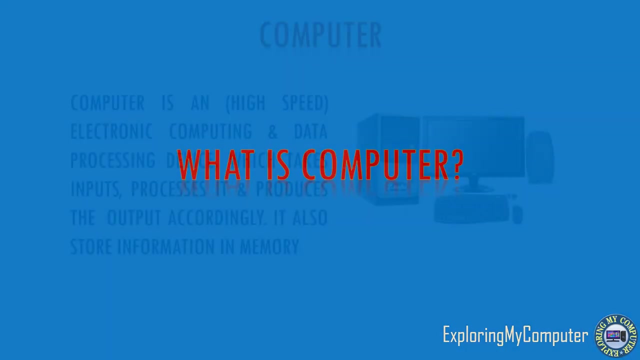 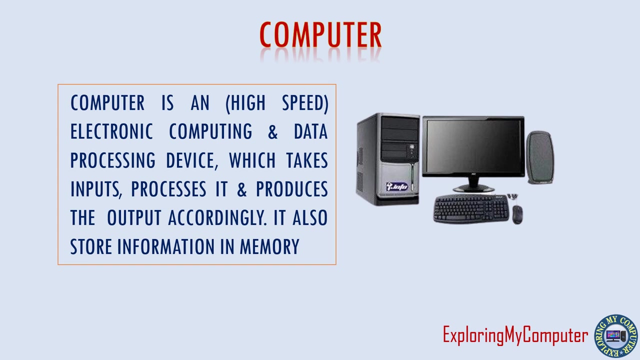 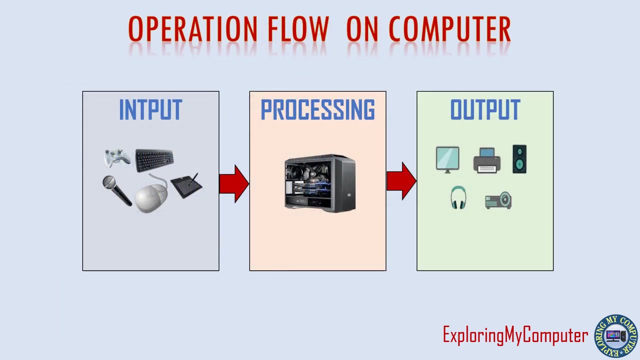 Welcome to Exploring My Computer Channel Watch videos on computer and solutions. Please stay connected by subscribing the channel for better, informative videos. Computer is an high speed electronic computing and data processing device which takes inputs, processes it and produces the output accordingly. It also store information in memory. 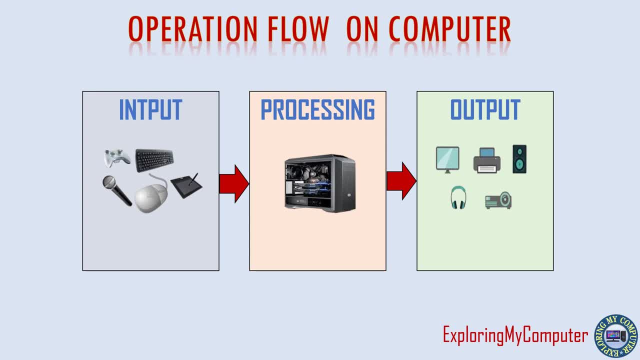 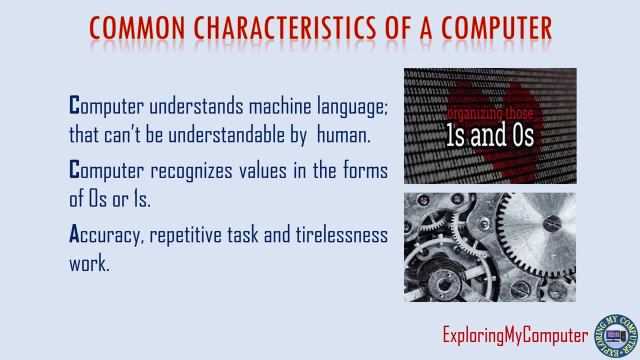 This diagram shows basic operation flow on computer, That is, input, processing and output. Common Characteristics of a Computer: Computer understands machine language that can't be understandable by human. Computer recognizes values in the forms of zeros or ones. Accuracy, repetitive task and tirelessness. 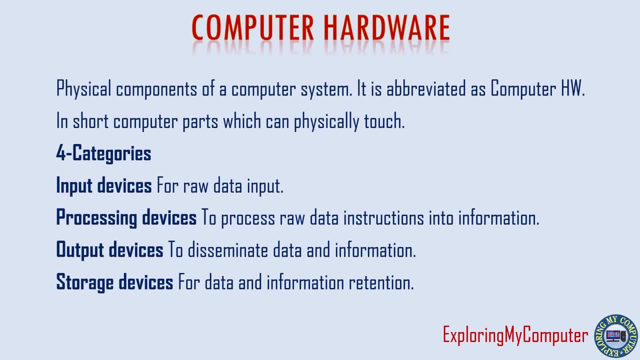 work. Computer Hardware is physical components of a computer system. It is abbreviated as Computer HW or HW In short, computer parts which can physically touch Four Categories: Input Devices for Raw Data. Input Processing Devices to process raw data instructions into information. Output Devices to disseminate data and information. 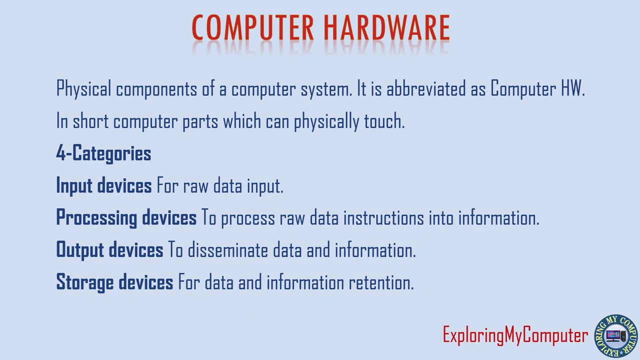 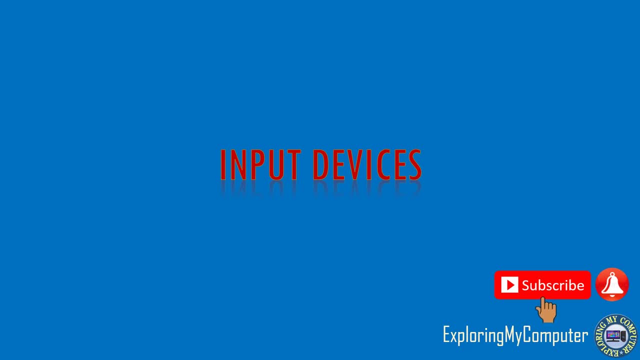 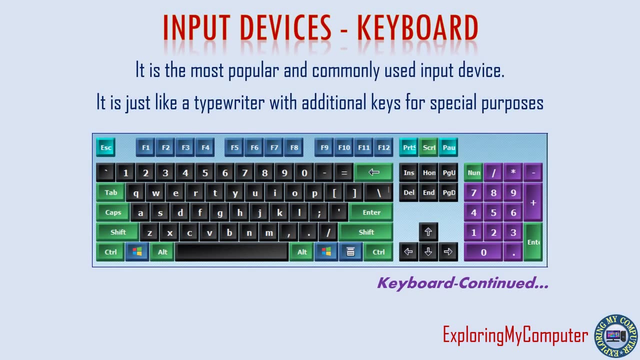 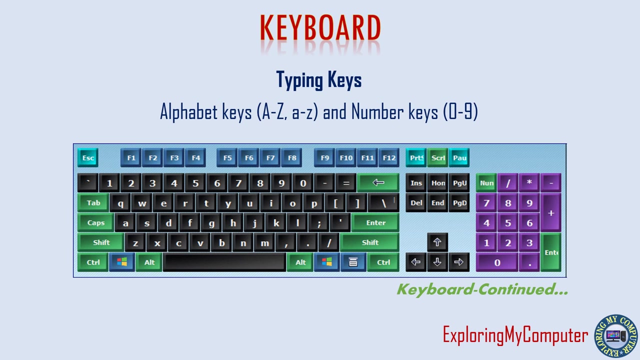 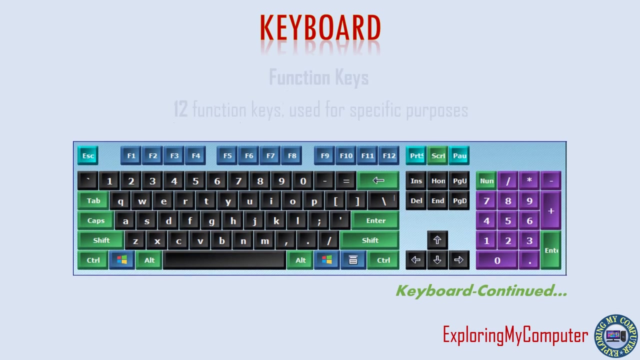 Storage Devices for data and information retention. Input Devices- Keyboard: It is the most popular and commonly used input device. It is just like a typewriter with additional keys for special purposes. Typing Keys, Alphabet Keys and Number Keys. Function Keys: Twelve function keys used for specific purposes. 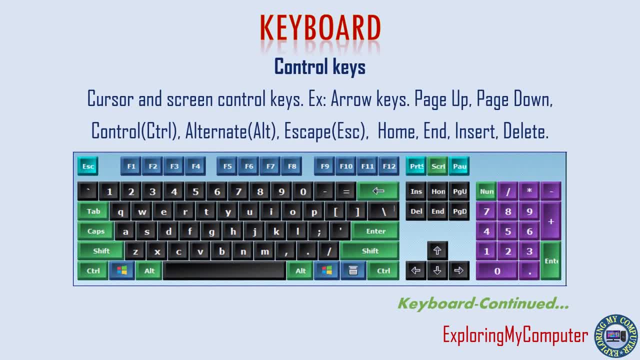 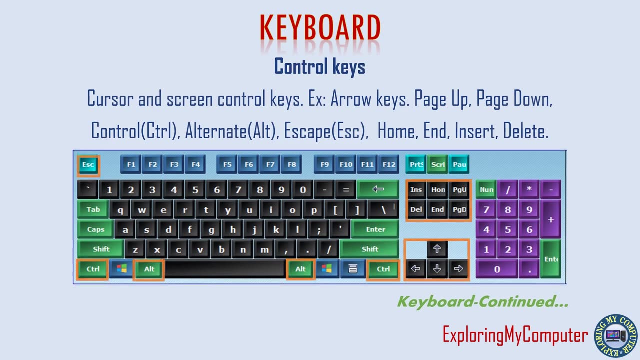 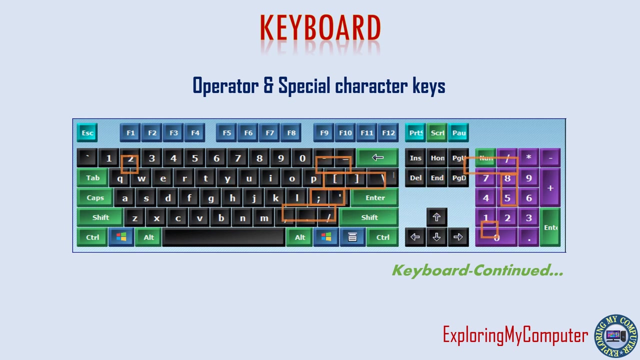 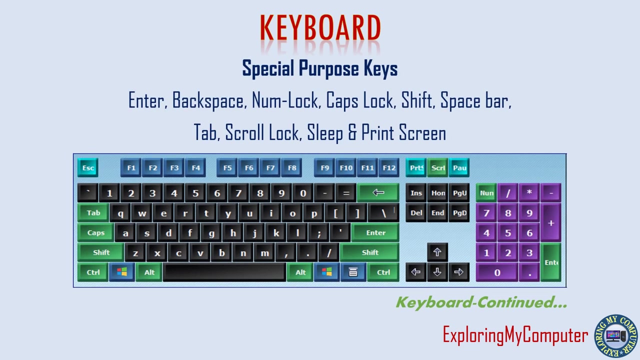 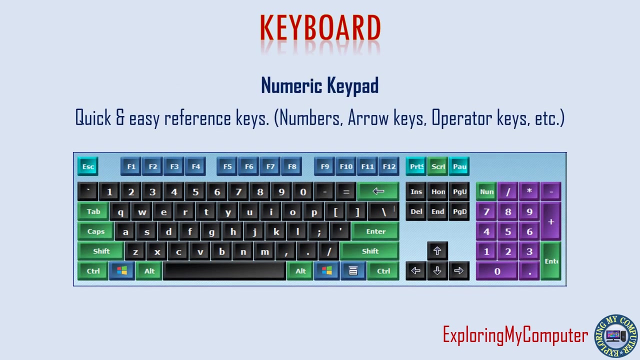 Control Keys. These are Cursor and Screen Control Keys. Example: Arrow Keys, Page Up, Page Down Control, Alternate, Escape, Home End, Insert and Delete Operator and Special Character Keys. alted while Control accessing Special Purpose Keys- Enter, Backspace, Numlock, Caps Lock, Shift, Space bar, Tab, Scroll Lock, Sleep and Print Screen Numberic Keypad. Quick and Easy Reference Keys, numbers, arrow keys, operator keys. 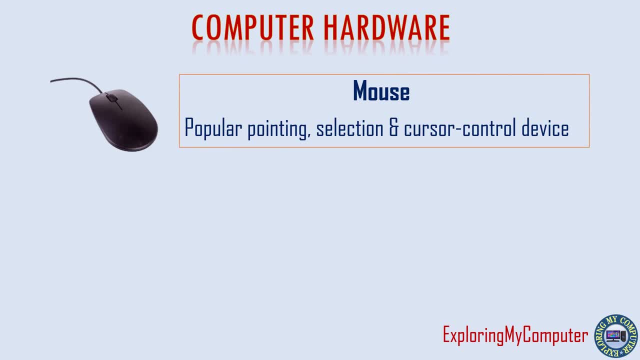 his-it-ter Manchester mouse. popular pointing, selection and cursor control dish, wakeacey, reference keys, numbers, arrow keys, operator keys, etc. feature reoccur עם a 세미் power key 돼 device microphone. it is used to recording sound, then stored in the 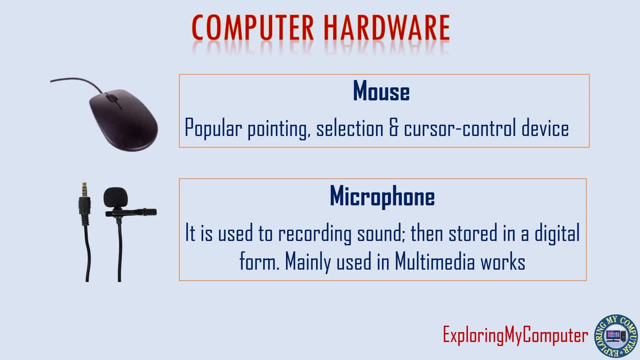 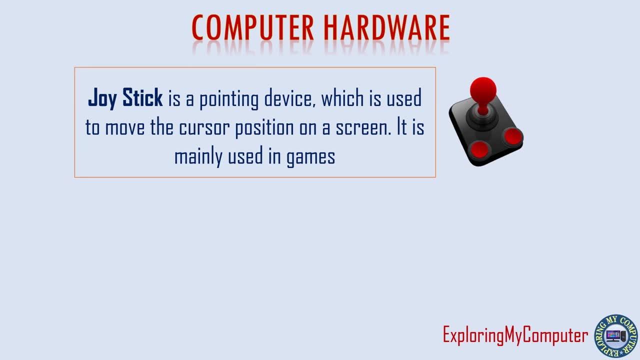 digital form mainly used in multimedia works. joystick is also a pointing device which is used to move the cursor position on a screen. it is mainly used in games. light pen is a pointing device similar to a pen, used to select a menu item or draw pictures on the screen. 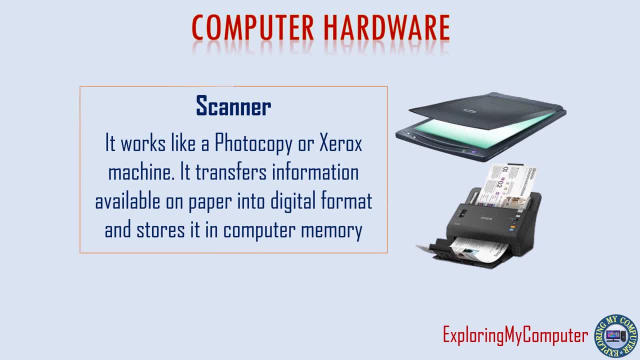 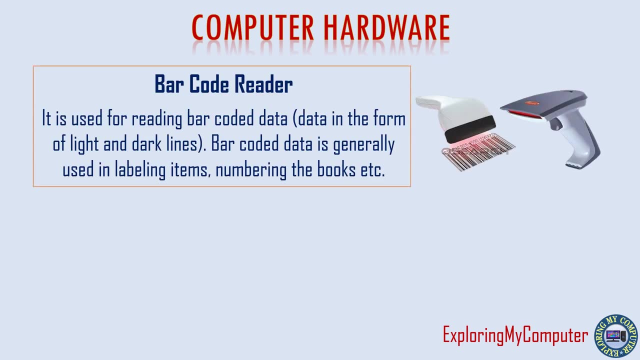 scanner. it works like a photocopy or xerox machine. it transfers information available on paper into digital format and stores it in computer memory. barcode reader: it is used for reading barcoded data data in the form of light and dark lines. barcoded data is generally used in labeling items. 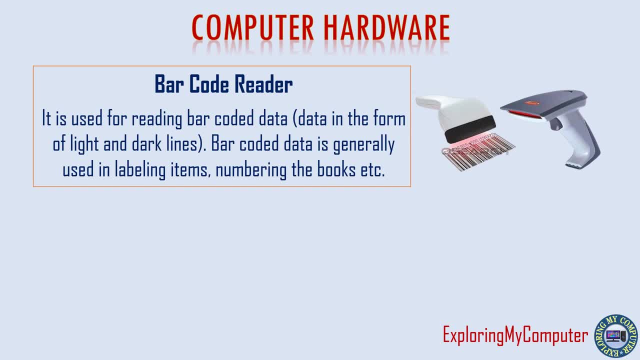 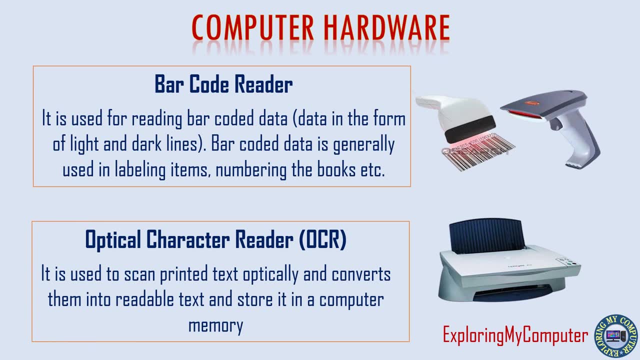 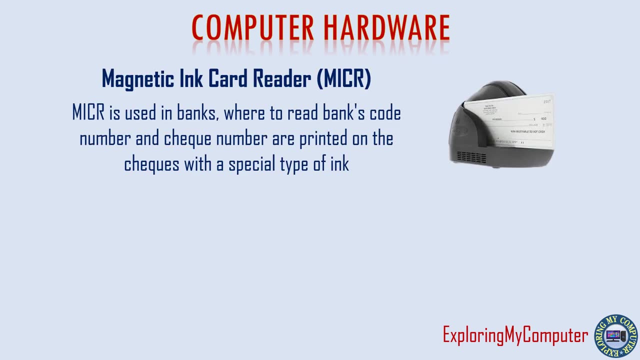 numbering the books, etc. optical character reader- OCR. OCR is used to read data in the form of light and dark lines, in the form of it is used to scan printed text optically and converts them into readable text and store it in a computer memory. magnetic ink card reader- MICR- is used in banks where to read banks. 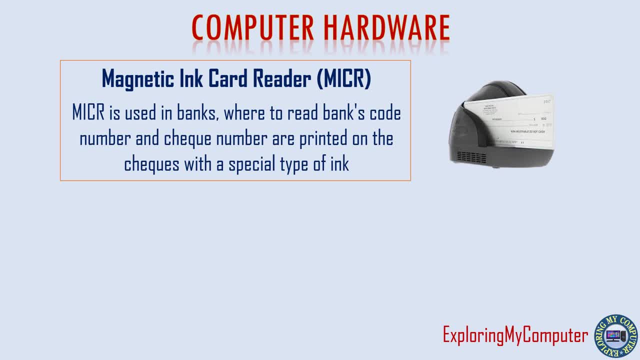 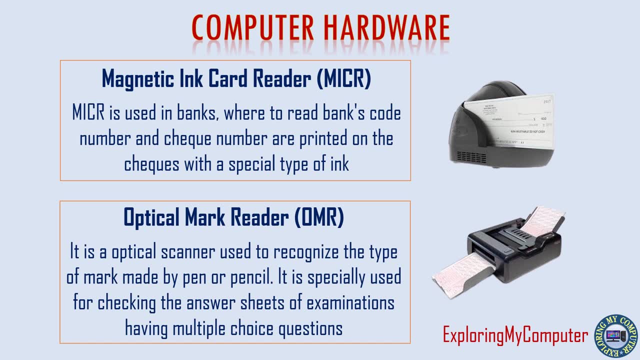 code number and check number are printed on the checks with a special type of ink optical mark reader, OMR. it is a optical scanner used to recognize the type of mark made by pen or pencil. it is special because it is used to scan printed text. OCR is especially used for checking the answer sheets of examinations having 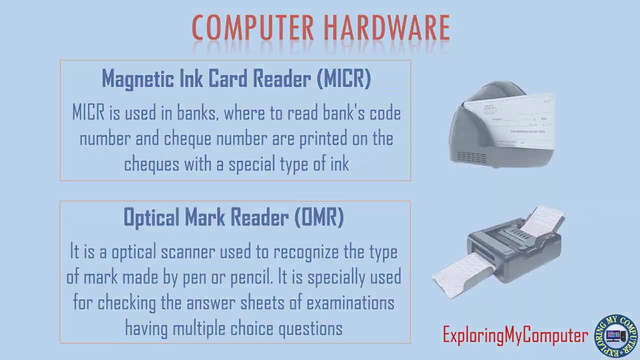 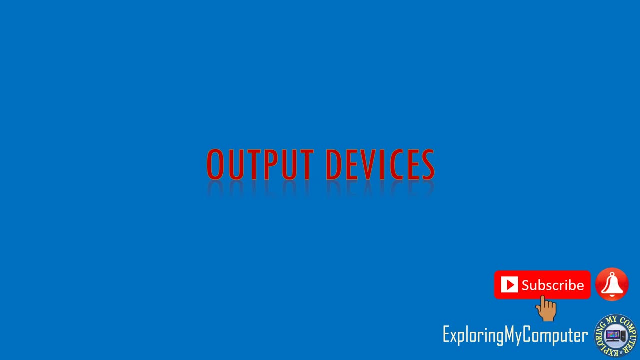 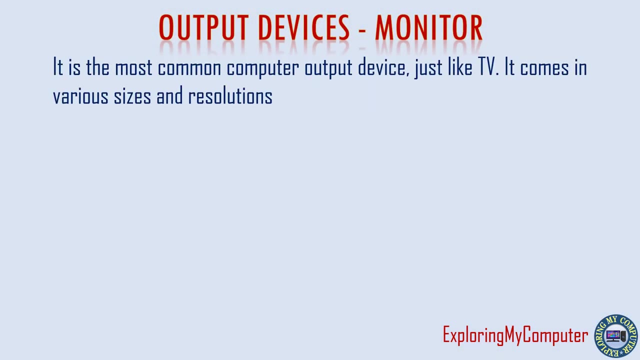 multiple-choice questions. you, you, you. you monitor the most common computer output device, just like TV. it comes in various sizes and resolutions. monitor resolution: it describes the visual display resolution connector is used for a monitor display dimensions of any given display Expressed in terms of width and height. monitor resolution: 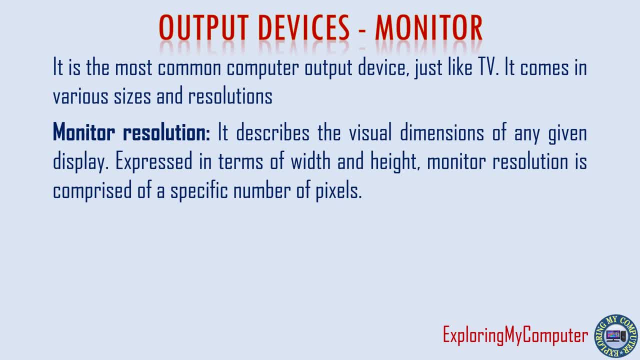 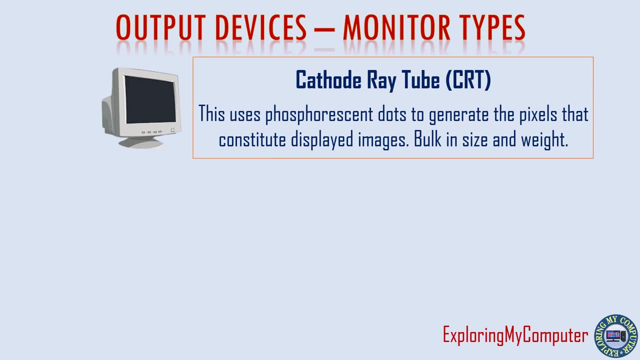 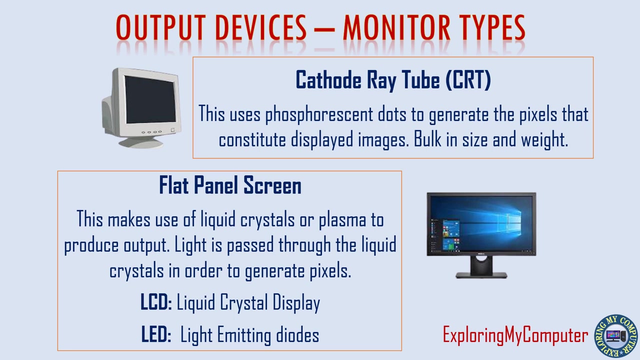 is comprised of a specific number of pixels. CRT cathode ray tube: This uses phosphorescent dots to generate the pixels that constitute displayed images. Bulk in size and weight. Flat panel screen: This makes use of liquid crystals or plasma to produce output Light. 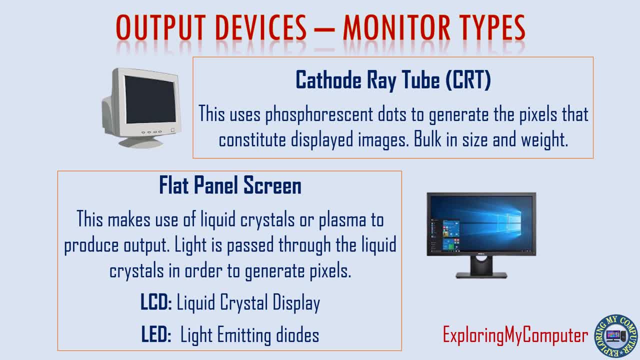 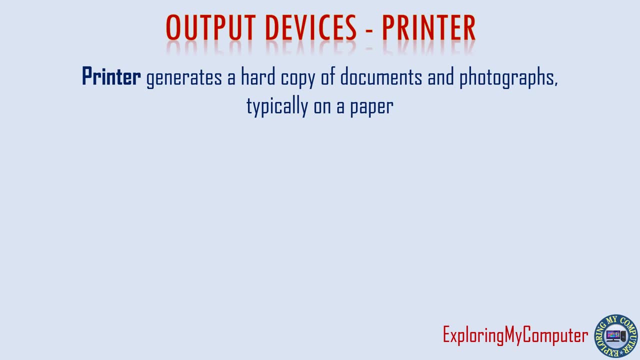 is passed through the liquid crystals in order to generate pixels. LCD. liquid crystal display. LED light emitting diodes Printer generates a hard copy of documents and photographs, typically on a paper. Impact printers works by direct contact of an ink ribbon with paper. 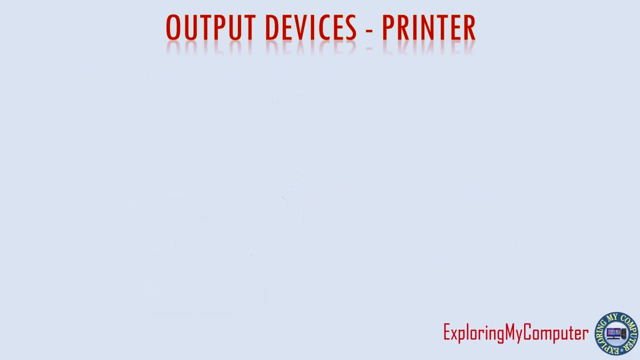 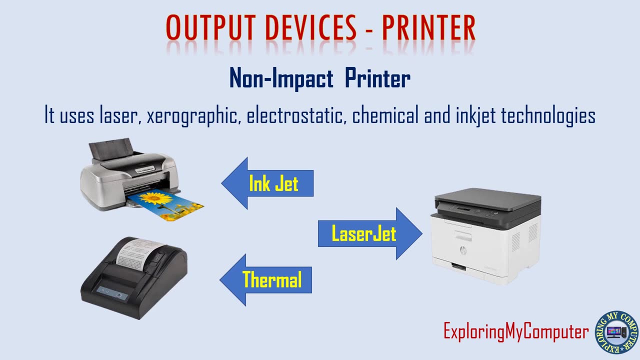 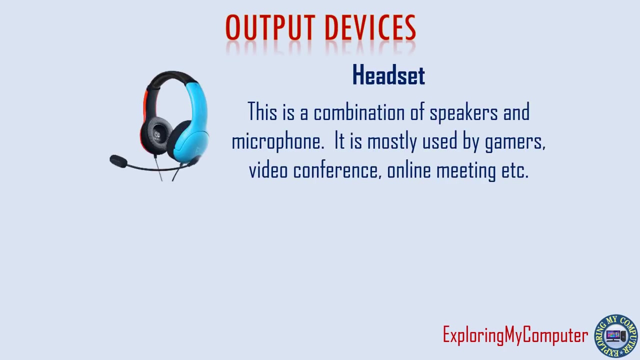 Non-impact printer uses laser, xerographic, electrostatic, chemical and inkjet technologies. Headset is a combination of speakers and microphone. It is mostly used by gamers, video conference, online meeting, etc. Speakers are to facilitate the output of digital sound. 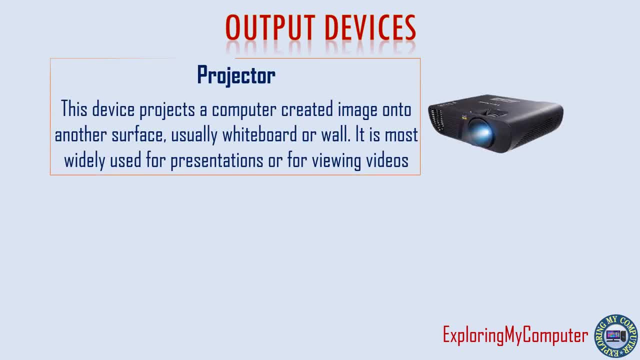 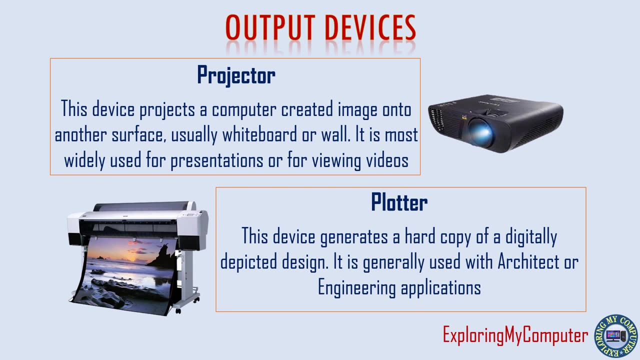 Projector device projects a computer created image onto another surface, usually whiteboard or wall. It is most widely used for presentations or for viewing videos. Plotter device generates a hard copy of a digitally depicted design. It is generally used with architect or engineering applications. 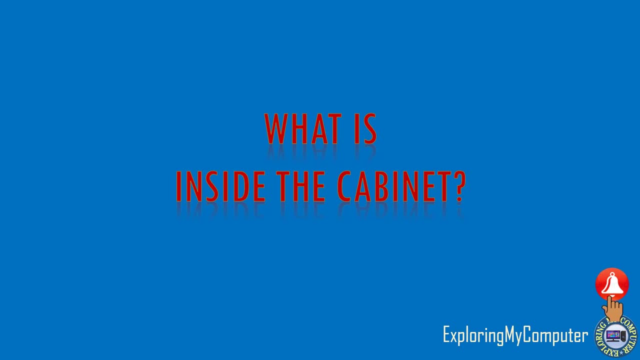 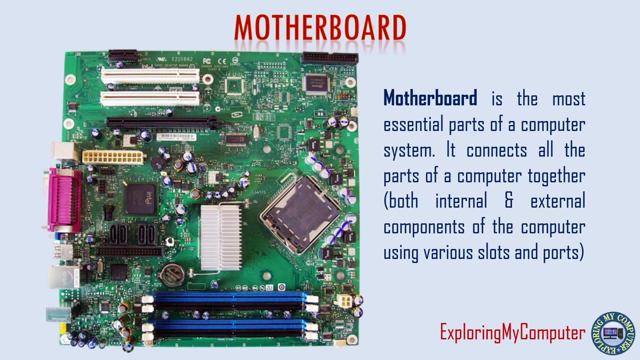 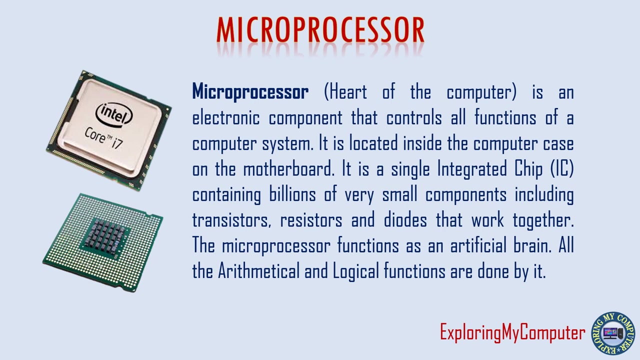 A VRS model 차�. Parts of a Computer System: sempre Doors, Back Keyboard, yse component that controls all functions of a computer system. It is located inside the computer case on the motherboard. It is a single integrated chip IC containing billions of very small 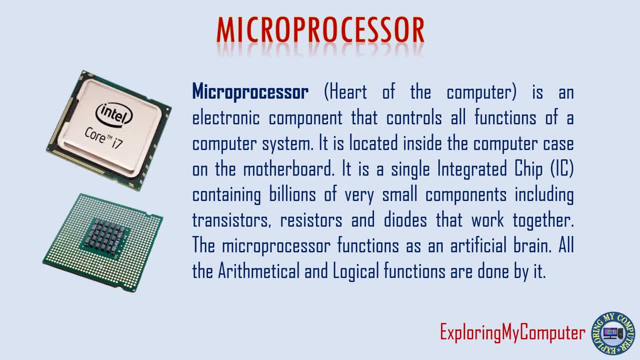 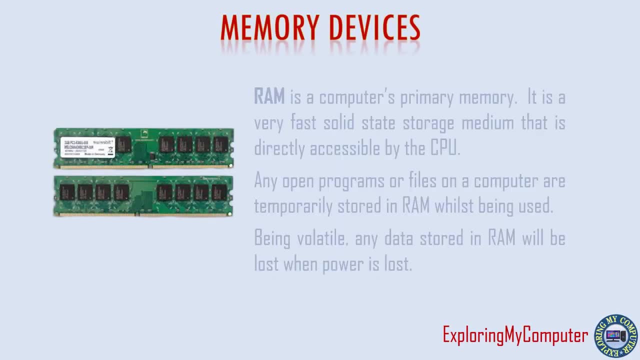 components, including transistors, resistors and diodes that work together. The microprocessor functions as an artificial brain. All the arithmetical and logical functions are done by it. Random access memory- RAM, is a computer's primary memory. It is a very fast, solid state storage. 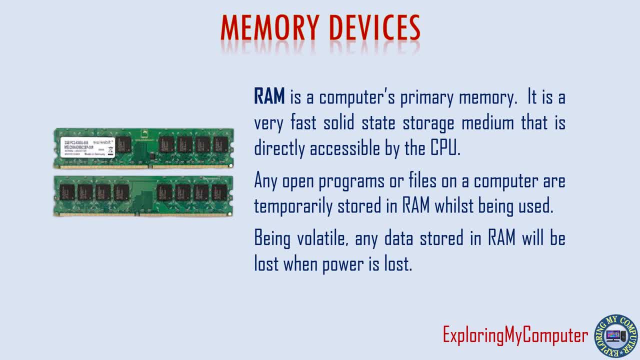 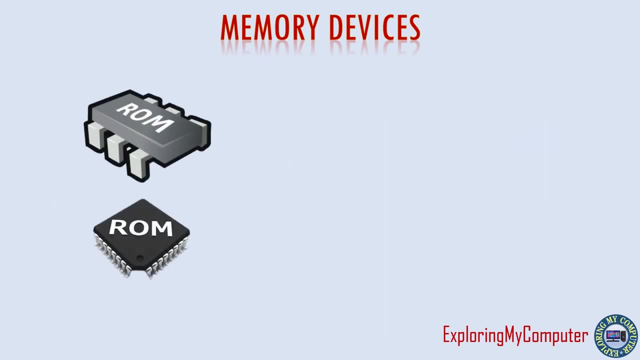 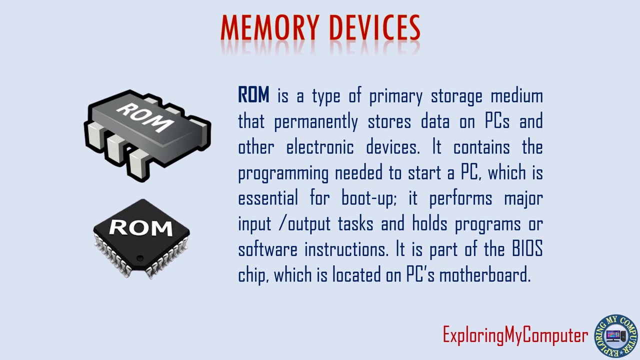 medium that is directly accessible by the CPU. Any open programs or files on a computer are temporarily stored in RAM whilst being used. Being volatile, any data stored in RAM will be lost when power is lost. Read-only memory ROM is a type of primary storage medium that permanently stores data on PCs and 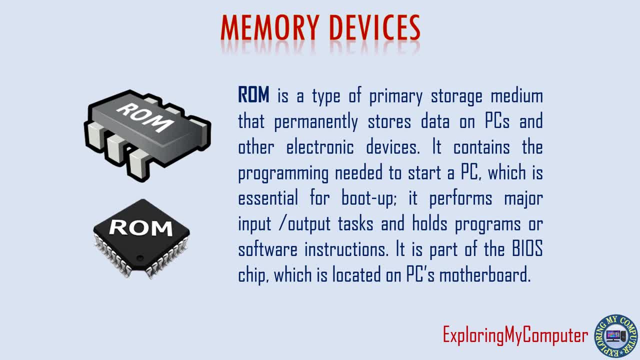 other electronic devices. It contains the programming needed to start a PC, which is essential for boot up. It performs major input-slash-output tasks and holds programs or software instructions. It is part of the BIOS chip which is located on PC's motherboard. 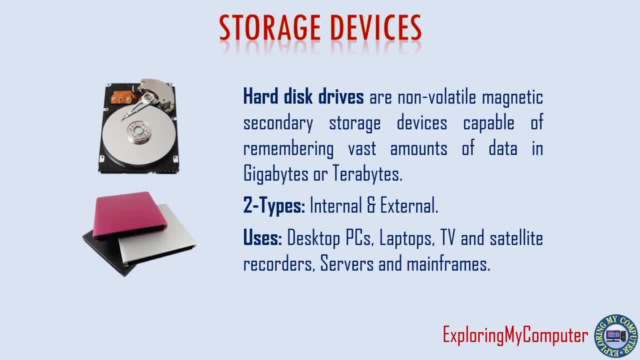 Hard disk memory Drives are non-volatile magnetic secondary storage devices capable of remembering vast amounts of data in gigabytes or terabytes. Two types: internal and external Uses: desktop PCs, laptops, TV and satellite recorders, servers and mainframes. 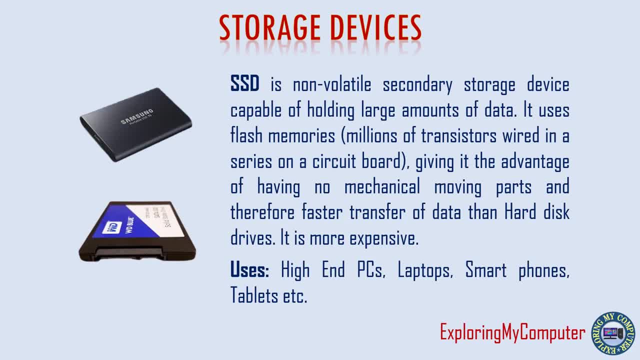 Solid-state drive. SSD is non-volatile secondary storage device capable of holding large amounts of data. It uses flash memory, Millions of transistors wired in a series on a circuit board, giving it the advantage of having no mechanical moving parts and therefore faster transfer of data than hard disk drives. It is more expensive. 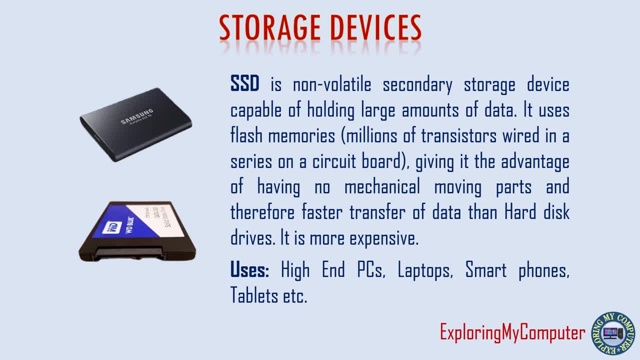 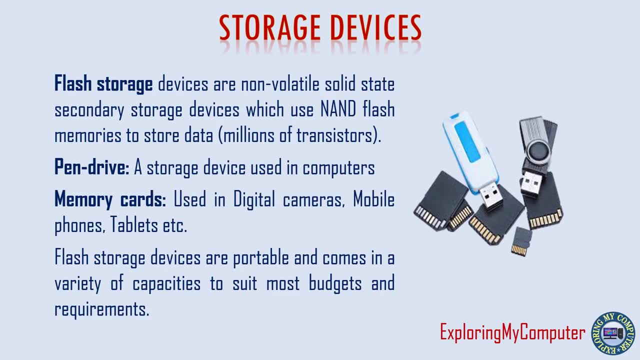 Uses high-end PCs, laptops, smartphones, tablets, etc. Flash storage devices. These are non-volatile solid-state secondary storage devices which use NAND flash memories to store data millions of transistors: pendrive used in computers, memory cards used in digital cameras, mobile phones, tablets, etc. flash storage devices are 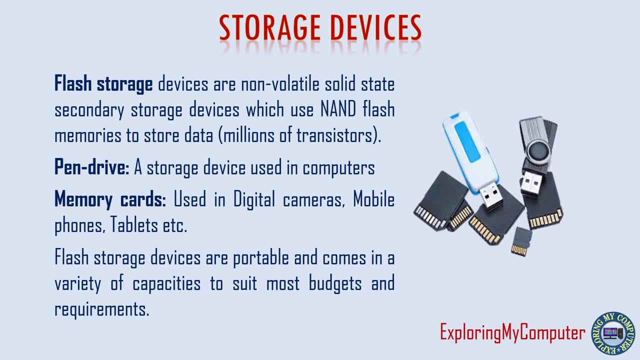 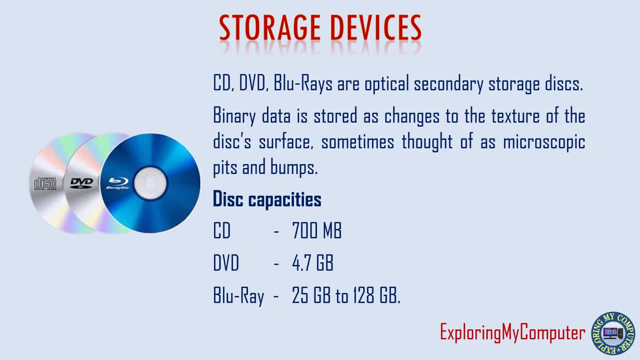 portable and comes in a variety of capacities to suit most budgets and requirements. CD- DVD blu-rays are optical secondary storage discs. binary data is stored as changes to the texture of the disc surface, sometimes thought of as microscopic pits and bumps. this capacity is: CD- 700 megabytes. DVD- 4.7 gigabytes. 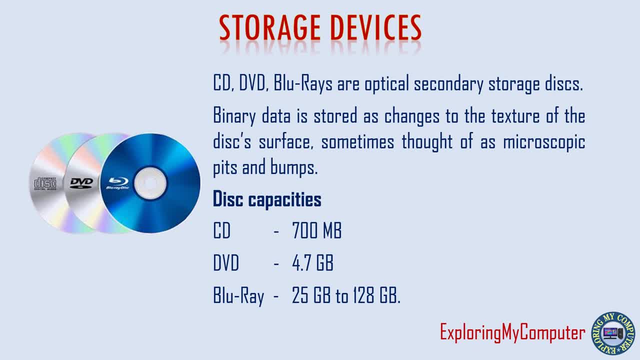 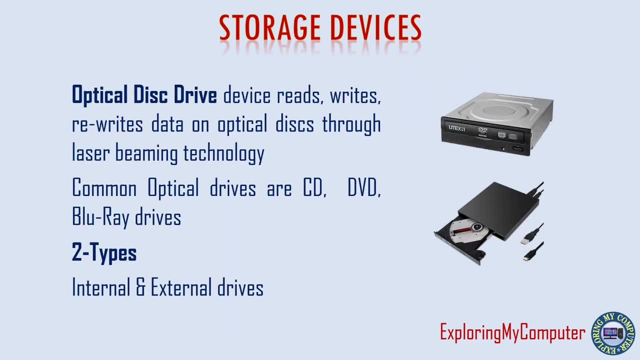 blu-ray, 25 gigabytes to 128 gigabytes optical disk drive. this device reads, writes, rewrites data on optical discs through laser beaming technology. common optical drives are: CD, DVD, blu-ray drives- two types: internal and external drives. CPU slot- the processor socket is the connector on the motherboard that. 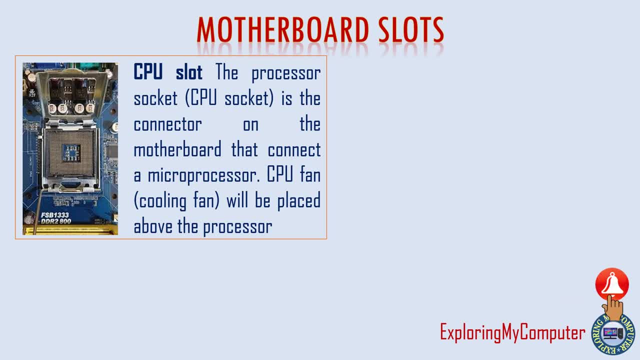 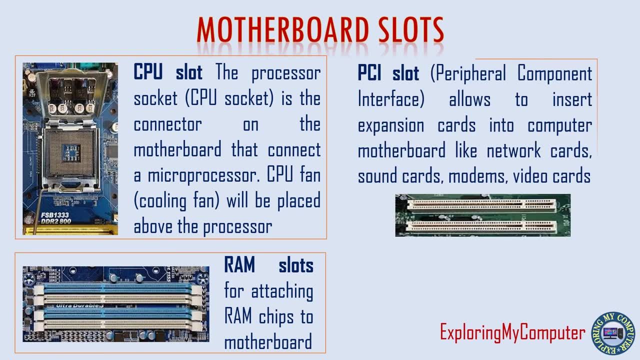 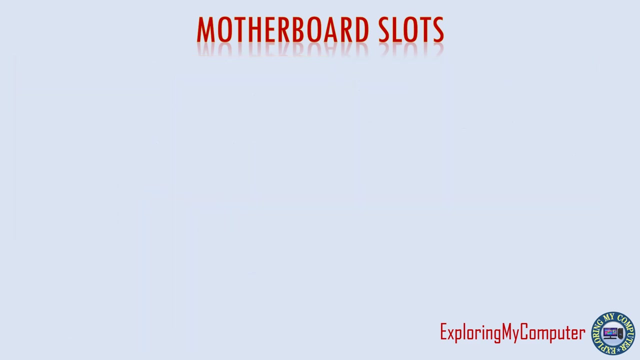 connect a microprocessor. CPU fan will be placed above the processor RAM slots. RAM slots for attaching RAM chips to motherboard, PCI slot. peripheral component interface slot allows to insert expansion cards into computer motherboard like network cards, sound cards, modems, video cards, AGP slot. Accelerated graphics port is a high speed point to point channel for attaching. 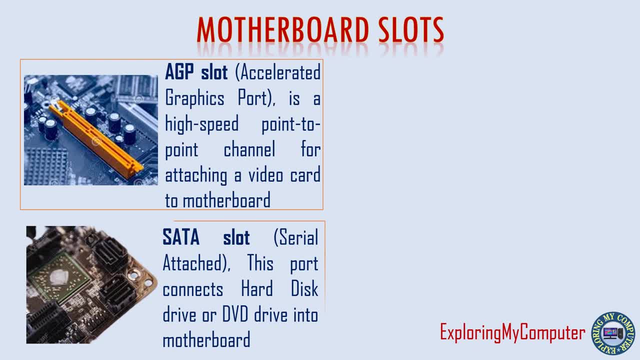 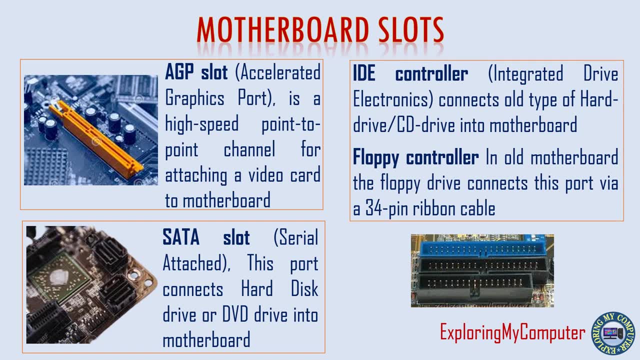 a video card to motherboard SATA Serial attached. this port connects hard disk drive or DVD drive into motherboard ID controller. Integrated drive electronics connects old type of hard drive or CD drive into motherboard Floppy controller. In old motherboard the floppy drive connects to computer via a 34. 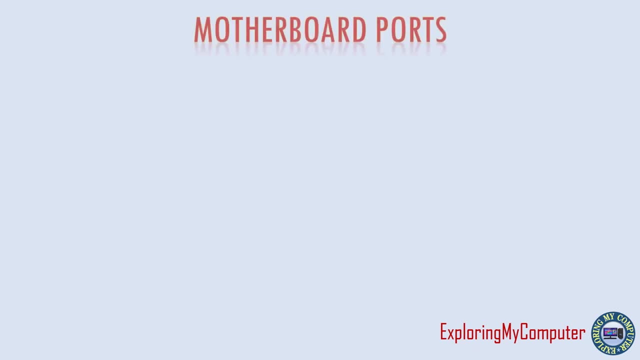 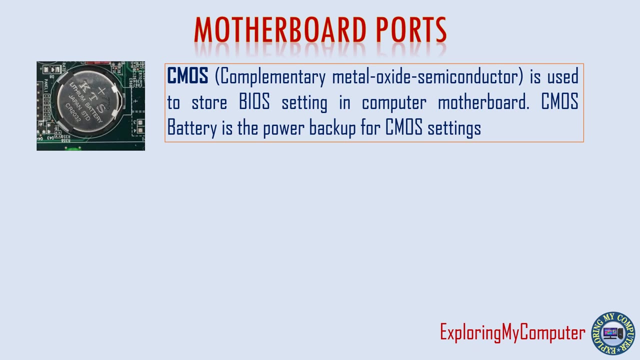 pin ribbon cable. CMOS battery. Complementary metal oxide semiconductor is used to stop IOS setting in computer motherboard. CMOS battery is the power backup for CMOS settings. PS2, Used to connect keyboard and mouse. USB Universal serial bus Used to connect mouse, keyboards, scanners. 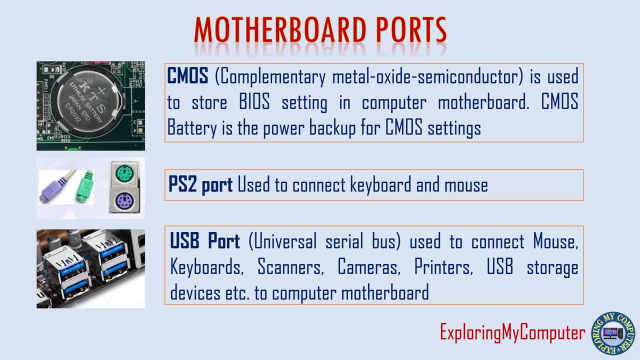 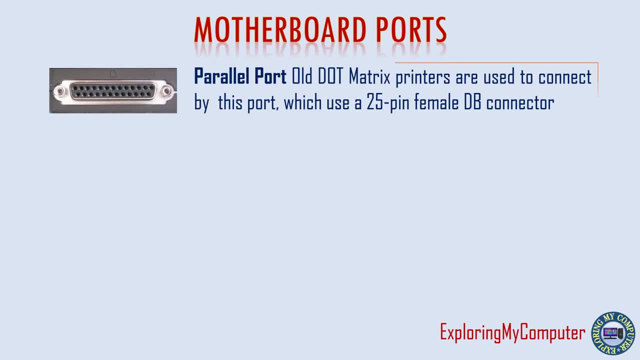 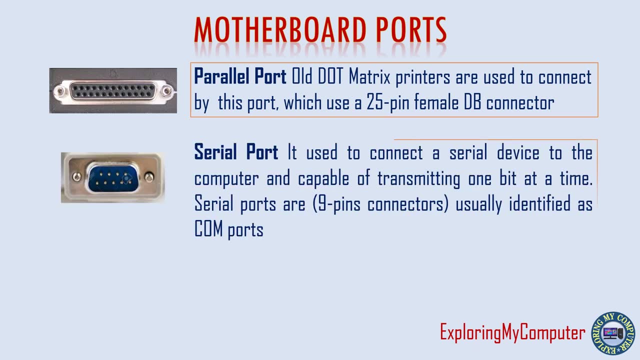 Cameras, printers, USB storage devices to computer motherboard. Parallel connector: Old printers are used to connect by parallel port which use a 25 pin female DB connector. Serial connector: It used to connect a serial device to the computer and capable of transmitting. 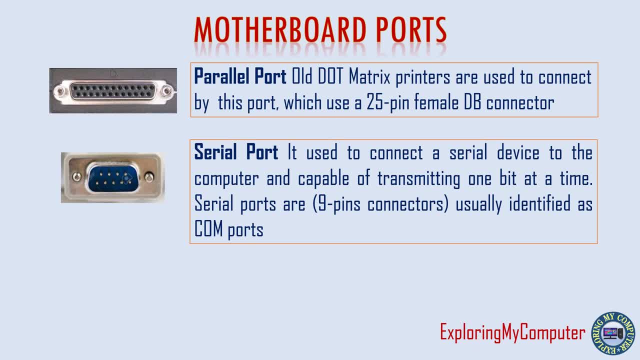 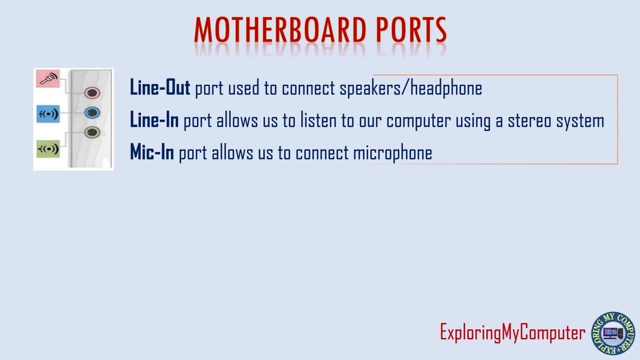 one bit at a time. Serial ports are 9 pins connectors, usually identified as COM ports. VGA Video graphics adapter Used to connect monitor into the video port Line out. It used to connect speakers or headphone into the line out jack. 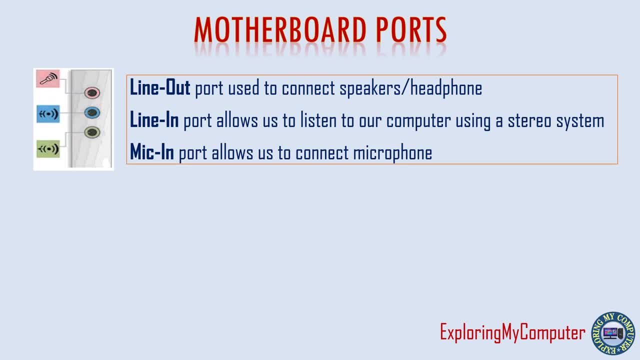 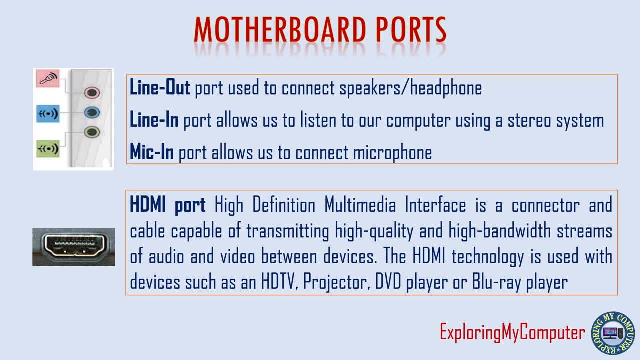 Line in The line in jack allows us to listen to our computer using a stereo system. HDMI High definition multimedia interface is a connector and cable capable of transmitting high quality and high bandwidth streams of audio and video between devices. The HDMI technology is used with devices such as an HDTV projector, DVD player or Blu-ray. 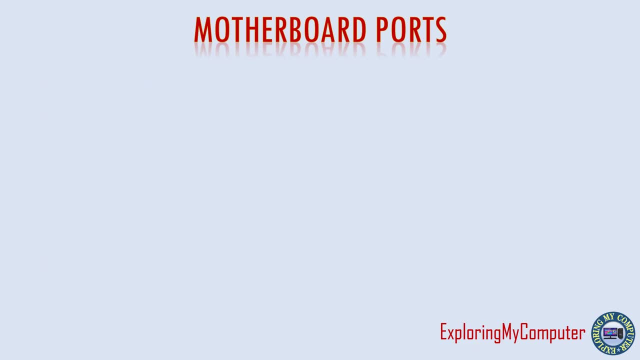 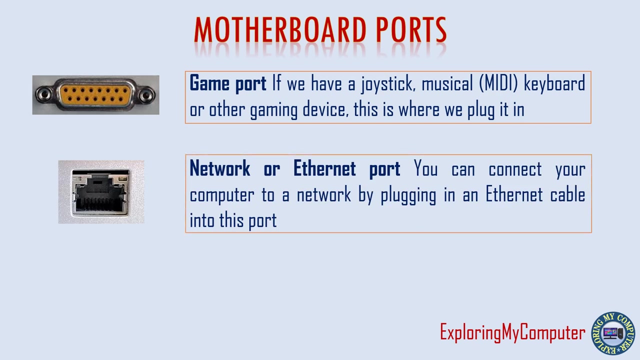 player Game port. If we have a joystick, musical midi keyboard or other gaming device, this is where we plug it in Network or Ethernet port. You can connect your computer to a network by plugging in an Ethernet cable in this port. 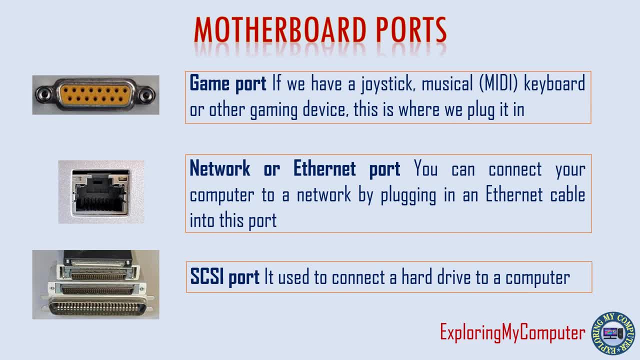 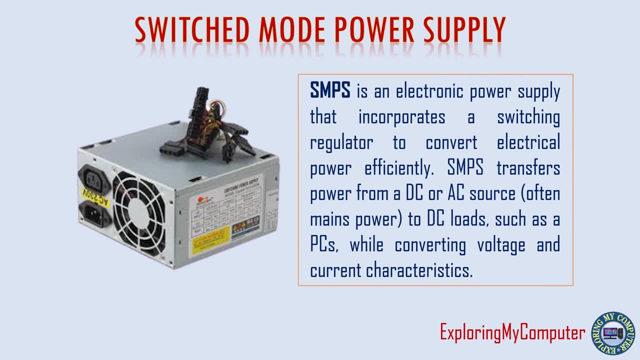 SCSI. This is where we plug in an Ethernet cable into a computer Switching Mode Power Supply. SMPS is an electronic power supply that incorporates a switching regulator to convert electrical power efficiently. SMPS transfers power from a DC or AC source, often mains power, to DC loads such as a.